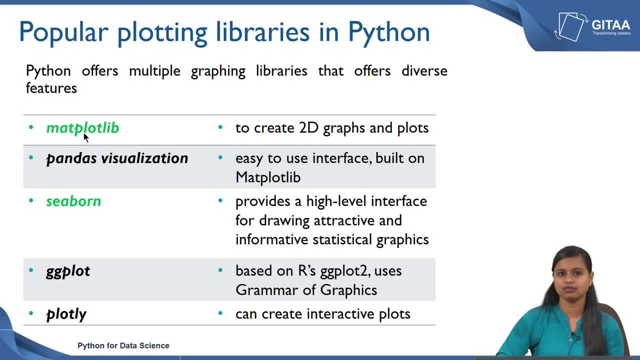 First one is matplotlib, which is used to create 2D graphs and plots, And I have marked it as screen because we are going to look at matplotlib library in this lecture. The next one is pandas visualization, which has easy to use interface and that was built. 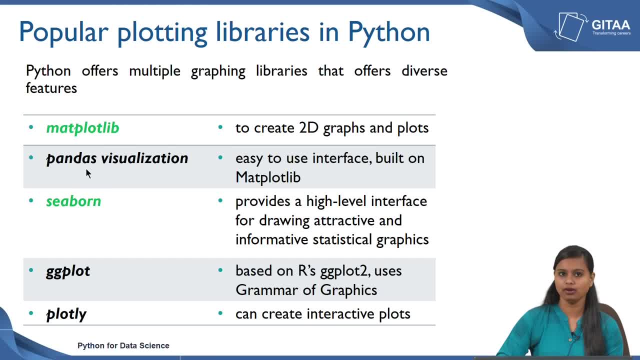 on top of matplotlib. The next one is seaborn. it provides a high level interface for drawing attractive and informative statistical graphics, and that was also built on top of matplotlib. Whatever graph and plots that you are creating using seaborn library can also be created using matplotlib. 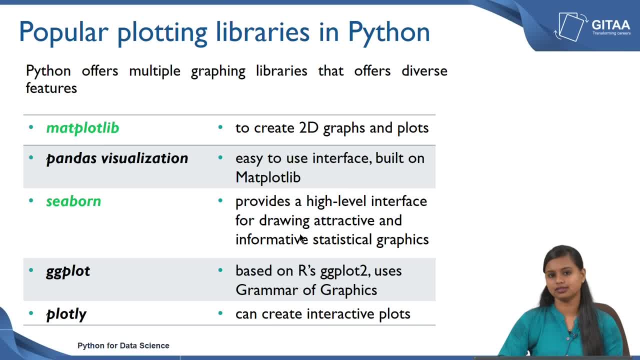 And you can also have a control on what insights you can get out of your plot using seaborn. The next one is ggplot. ggplot is used whenever you want to do a advanced graphics, and this ggplot is entirely based on R's ggplot. R is another programming language that is used. 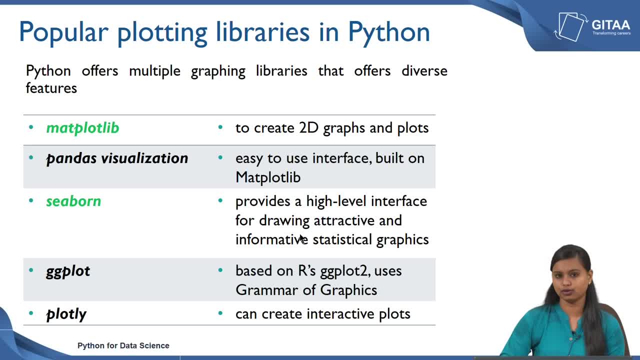 for analytics and it has a package called ggplot2 which is entirely dedicated for doing visualization In python. we have ggplot that is based on R's ggplot2 and it basically uses grammars of graphics. The next is plotly. if you want to create interactive plots, then you can go for plotly. 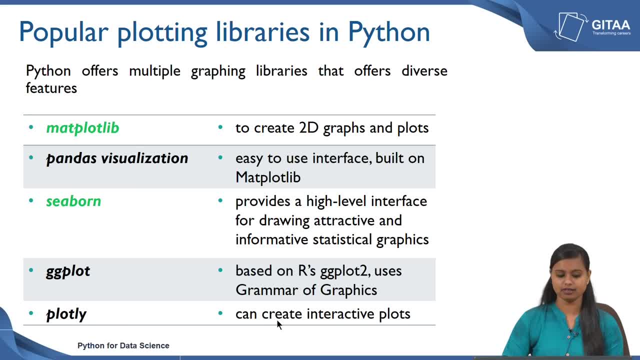 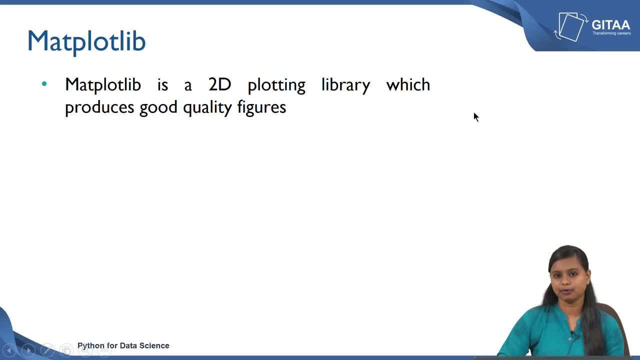 But in this course we are going to look at two graphing libraries that are matplotlib and seaborn. First we are going to look at a matplot library. So let us see what matplot library is about. matplot library is a 2D plotting library, which 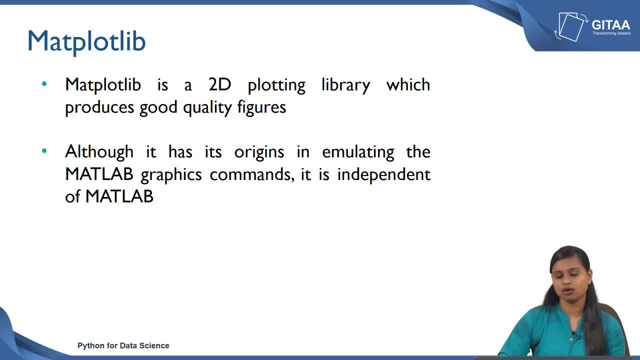 produces good quality feedback. It has a lot of features. although it has its origin in emulating the matlab graphic commands, it is independent of matlab. It makes heavy use of numpy and other extension code to provide good performance even for large arrays. So this is the overview of the matplotlib library. 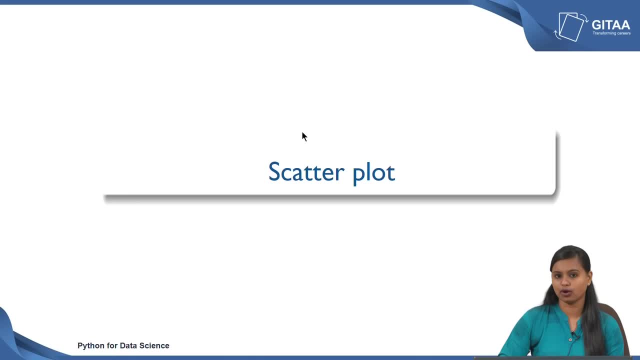 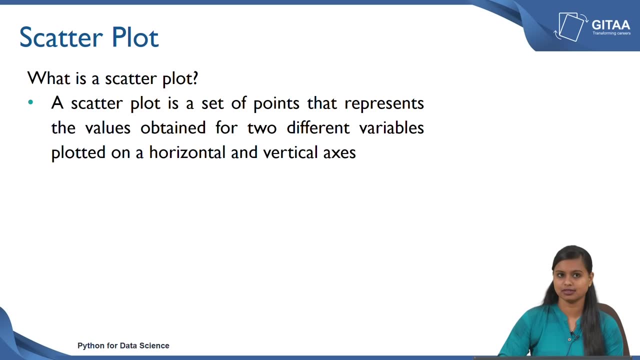 So under the matplotlib library we are going to look at a plot called scatterplot. So let us see what is the scatterplot first. A scatterplot is basically a set of points that represents the values that obtained for two different variables, Plotted on a horizontal and vertical axis. 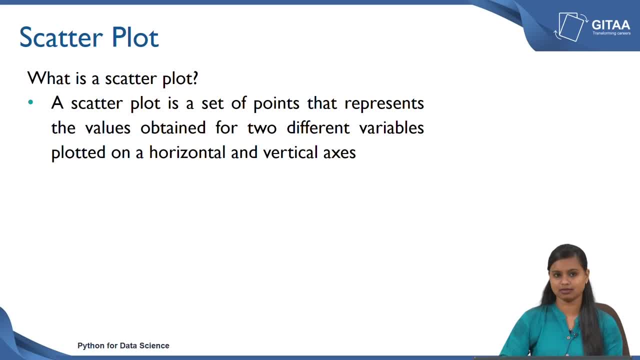 So, if you look at a scatterplot, you will have two axis toward x and y, and the points from the data frame will be scattered all over the place of the plot or in a separate pattern, and using that, and using the variables that you have given as an input, you will get 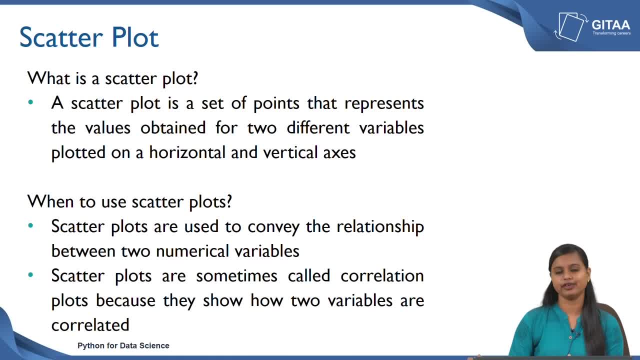 the relationship out of it and there can be a question when to use the scatterplots. So, basically, the scatterplots are used to convey the relationship between any two numerical variables, How one variable vary with respect to the other variable, and scatterplots are also sometimes 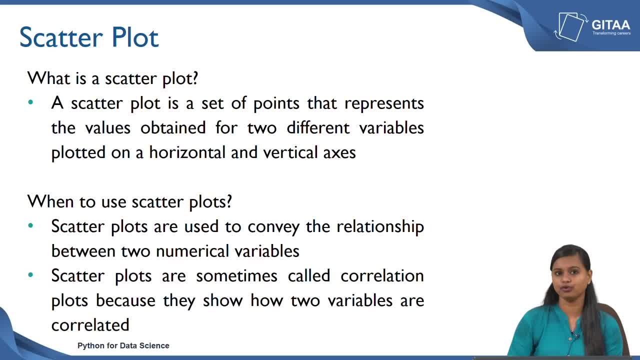 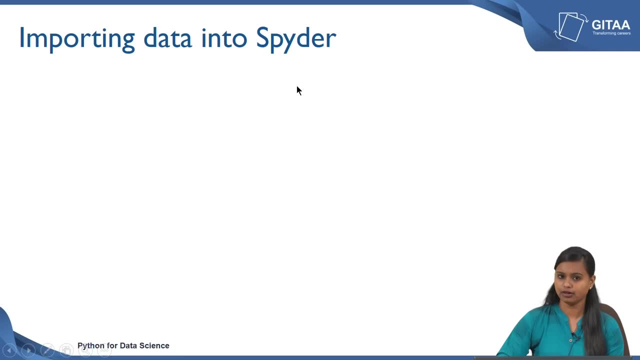 called as correlation plots, because they show how two variables are correlated, whether they are negatively correlated or positively correlated. all those information you can get that by looking at the patterns of your scatterplots. So now we are going to import the data into SPIRAL to do a scatterplot prior to importing. 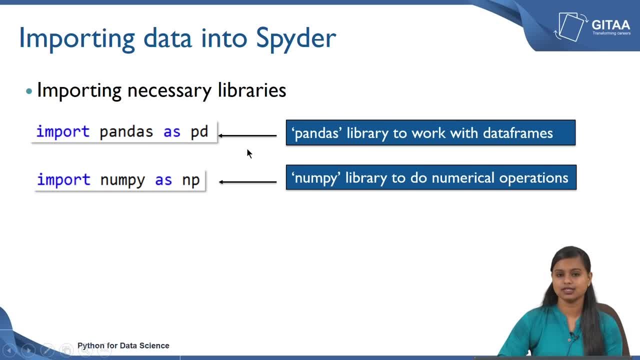 the data to import the necessary libraries. The first library is pandas and we have imported it with the alias pd and we have to import the pandas library to work with data frames and then we will also be doing some numerical operations on it. So we need to import numpy. 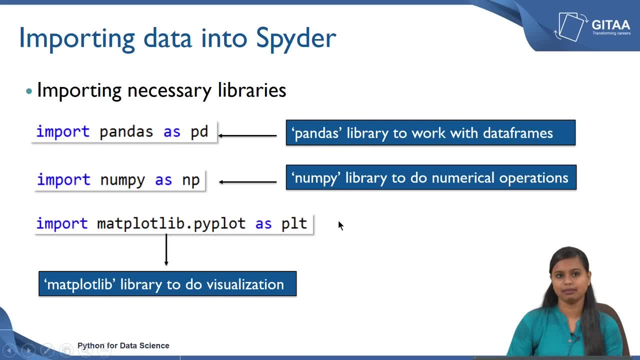 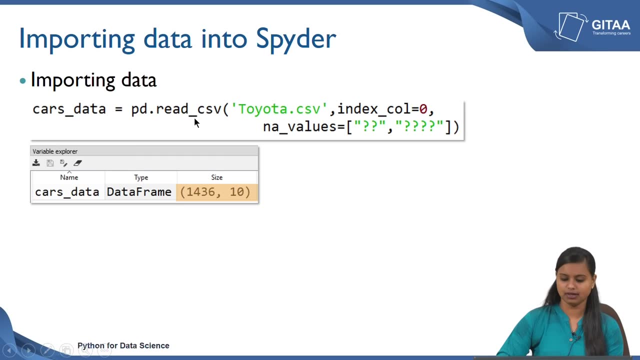 as np and then, since we are going to use the matplotlib library and we have to import pyplot from the matplotlib as plt and we use this to do visualization. Now we can import the data into spider using the read underscore csv command and we have set the first column as the index column and we have considered all the question marks. 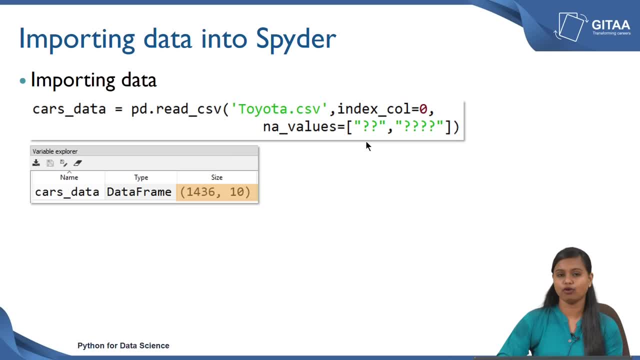 as default nan values so that we can do any operations that are related to nan values. So cars underscore data is your data frame now and the size of it is 1436 with 10.5 nan, 10 columns. We are going to remove all the missing values from the data frame because 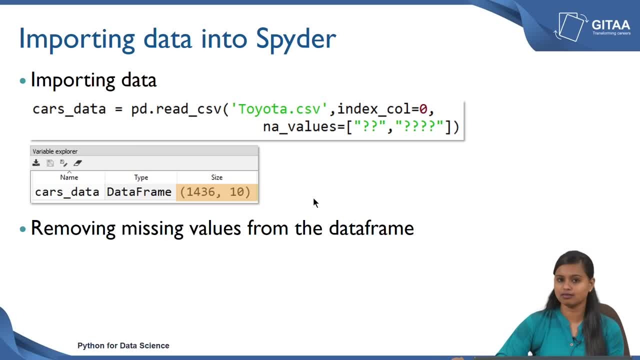 we are going to visualize the data. in that case, I do not want to consider all the missing values. rather, I just want to consider all the rows where there are no missing values. So in that case, if you want to drop out all the records where there are missing values, 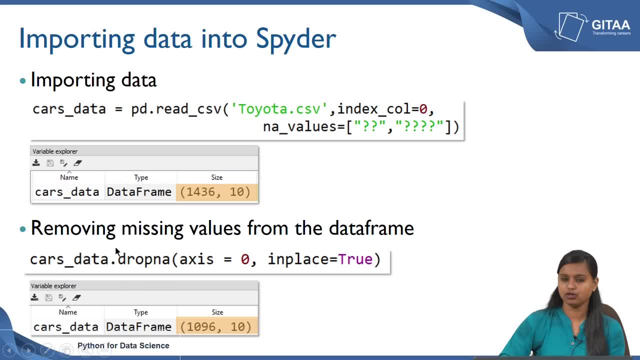 then you can use the command called drop, na preceded with the data frame name and inside the function, if you set, access is equal to 0. You consider all the rows where there are missing values and remove that I have also given in place is equal to true. that is because I have not assigned this to a new data frame. 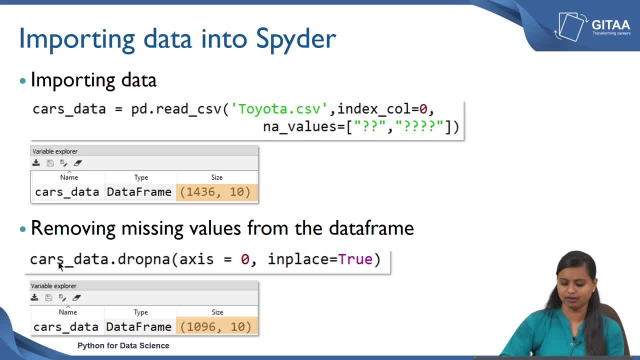 as cars underscore data 2 or or in the existing data frame. rather, I have just used in place is equal to true. by setting in place is equal to true, the modifications that you are making here will be reflected in the data. if you do not give this, the records will not be dropped. 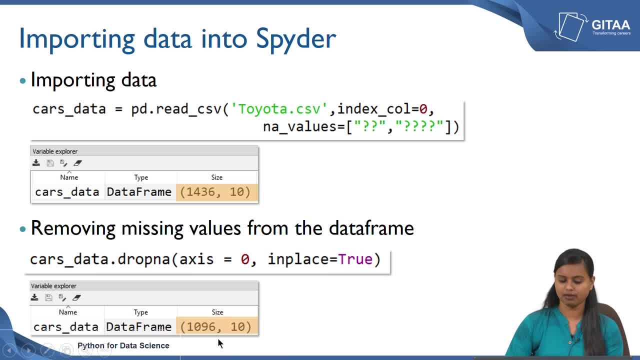 from your data frame. If you look at the size of your data frame after removing the missing values, it turned out to be having 1096 observations with 10 columns, So we have left out around 400 observations. So now let us see how to create a scatter plot. 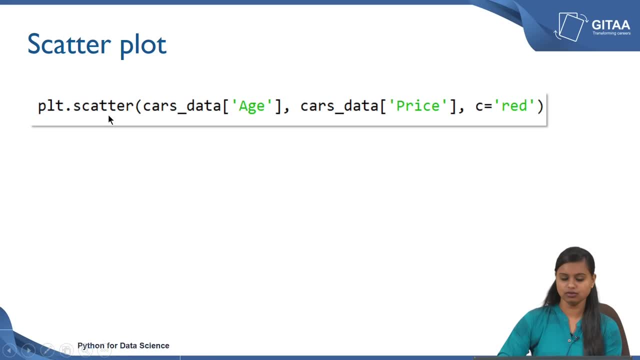 So for creating a scatter plot, scatter is the function. since we are doing it from the matplotlib library, we have saved piplot as plt, So that is why I have used the allies called plt to access the function scatter, and inside the function I have given the x coordinate variable, that is h, and I have also given the 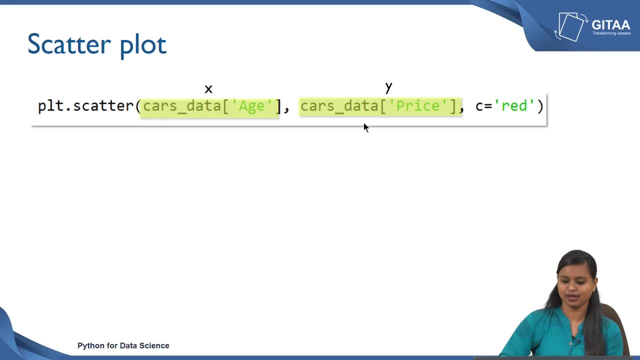 y coordinate variable, that is price. So it is very evident that we are going to check the relationship between age and price through scatterplot. And the next thing is I have given red under the parameter c. that means that I am going to color the markers using the red color. 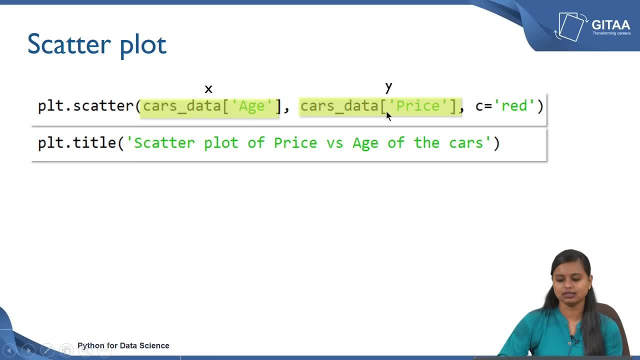 So we will see what marker is when we get the output. This line will produce a scatterplot, but if you want to add title to your plot and if you want to add labels to your x axis and y axis, you can also give that. 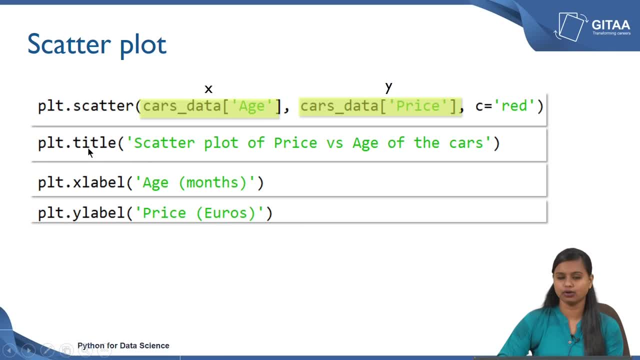 See, if you want to add title to your plot, you can give it as plt dot title and inside that I have just given it as scatterplot of prices. h of the cars, and the x label represents the age, which are in months, And the y axis represents the price, which are in euros. 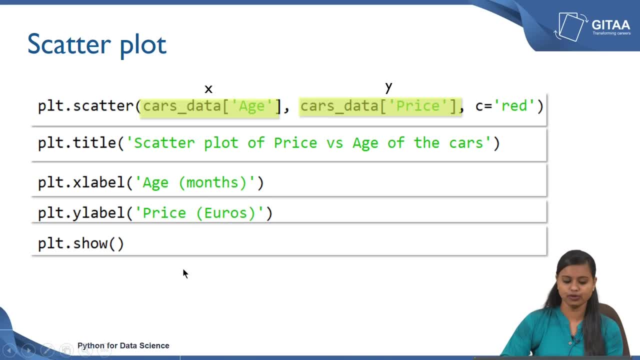 Now we have created a scatterplot. to show the scatterplot, you have to use plt dot show. Even if you select the lines to plt dot y label, you will be able to show the plot, since this is a standardized code. whenever you are building your plots layer by layer, by giving 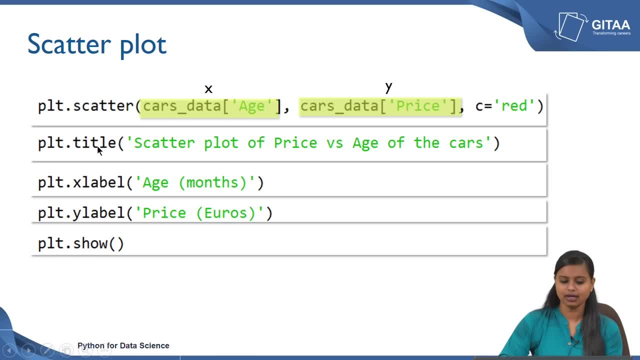 the type of plot first and then giving titles after that. then you have to run everything in one shot till plot dot show To get all the information in a single plot. So now let us see what is the output by using the scatter function. 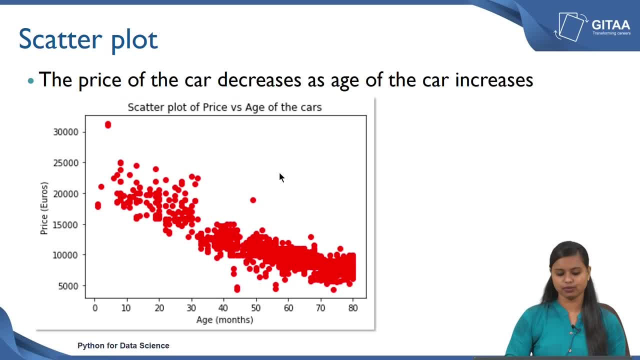 Here this is the scatterplot to show the relationship between price of the car and the age of the car. See, if you see from the output, your x axis represents the age and y axis represents the price. If you see here, as the age increases, the price decreases. 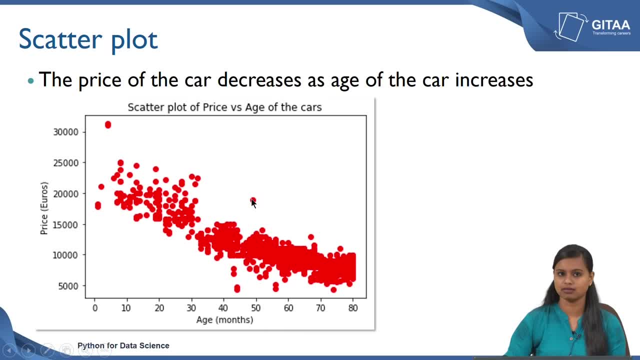 Yes, Yeah, shown here are called as markers and the vertical line that is shown here are ticks, and 60,, 70,, 80 are called tick labels. since these are in x axis, these are called x ticks and x labels and these lines are called y ticks and these values are called y tick labels. 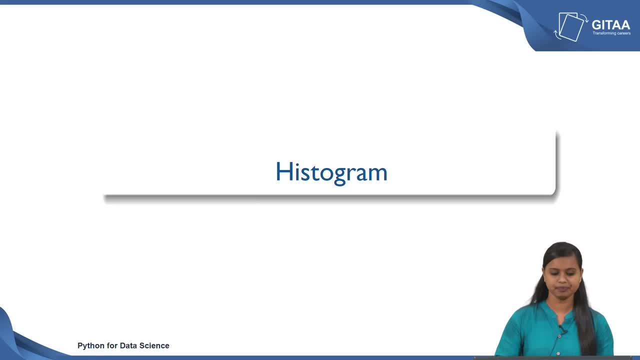 So now we are going to see how to create the histogram. Before creating, we need to know what histogram is. So what is a histogram? It is a graphical representation of data using bars of different heights. So whenever you have a numerical variable and if you want to check the frequency distribution, 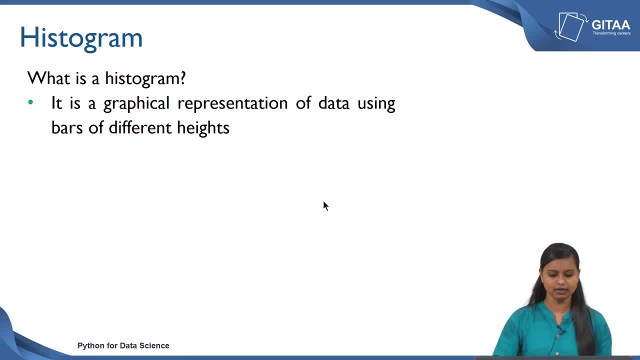 of the variables. you can go for histogram So that the each bar will give you different heights. that represents the frequencies, And the histograms groups numbers In two ranges, because on the x axis you will have intervals or ranges. that can also be. 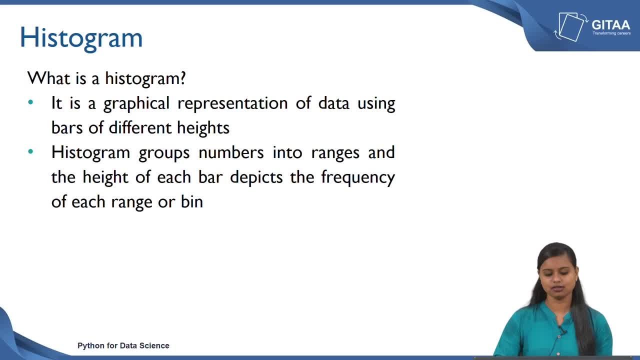 called as bins, And for each of the bins you will get a corresponding frequency by looking at the height of each bars. So when to use the histogram, as I have mentioned, to represent the frequency distribution of any numerical variables, you can look for histogram. 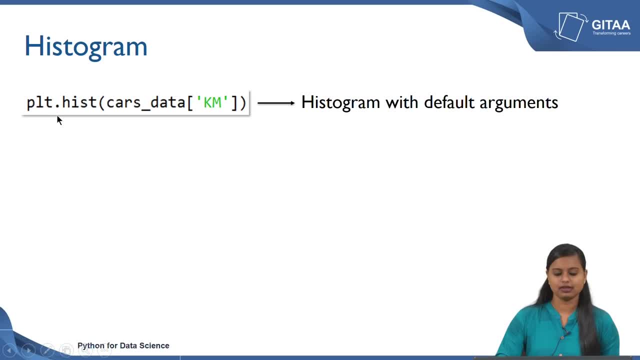 Now we will see how to create a histogram using matplotlib. So the command is hist, that stands for histogram And that is from the library called piplot, library called matplotlib, and piplot is the sub library that is available under matplot and pelt is just analyzed to the piplot. 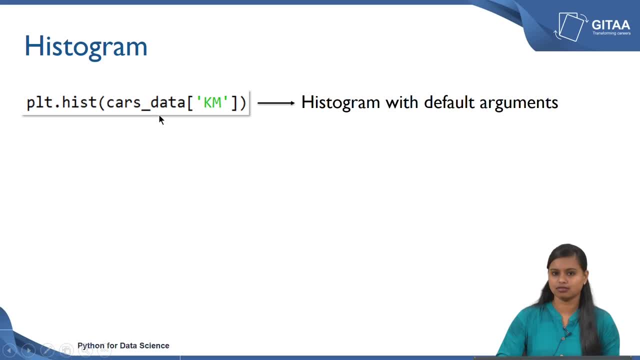 And inside the function I will just given kilometer from the cars, underscore data data frame. So that becomes the x axis. So we are creating a histogram with the default arguments because we have just given the x variable alone. And let us look at the output. 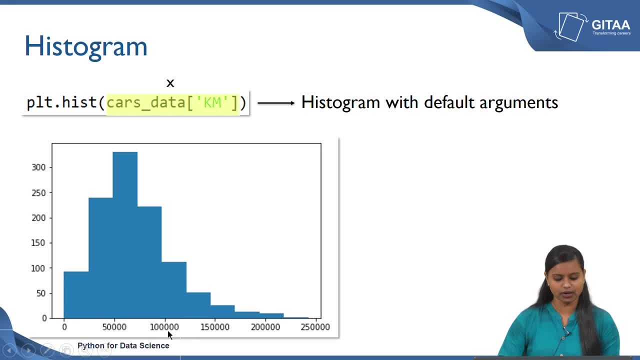 So here is the histogram with default arguments. on the x axis you have the bins. The first bin is from 0 to 50000, and the second bin is from 50000 1 to 1 lakh and the third bin is from 1 lakh 1 to 1 lakh 50000. 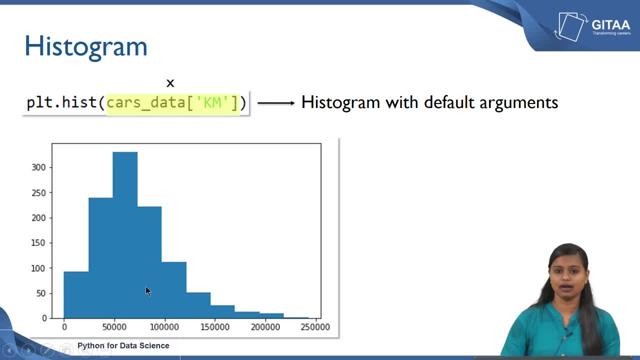 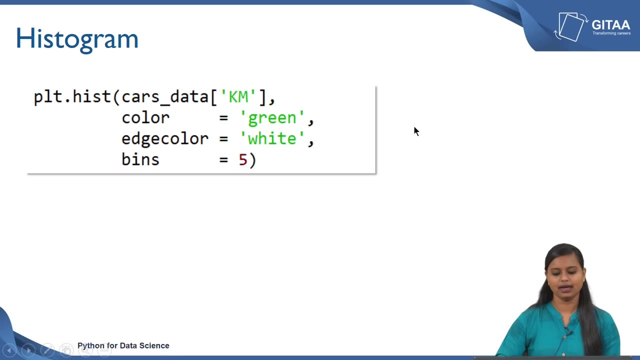 For example, using this histogram, I am not able to get the exact bin range or the exact range, the corresponding frequency, Because it does not Give me the separation between each bars. So now what I can do here is I can create a histogram by specifying the edge color and 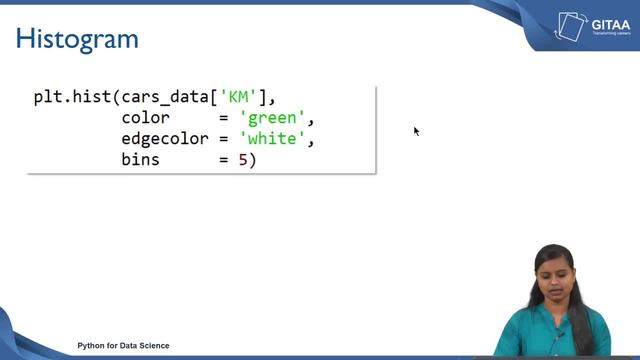 the number of bins I have. If I have too many bins, then it would not be able to easier for us to understand the frequencies for each interval. In that case you can specify or fix the number of bins as well. So here we are using the same command where we have fixed the x coordinate, that is, kilometer. 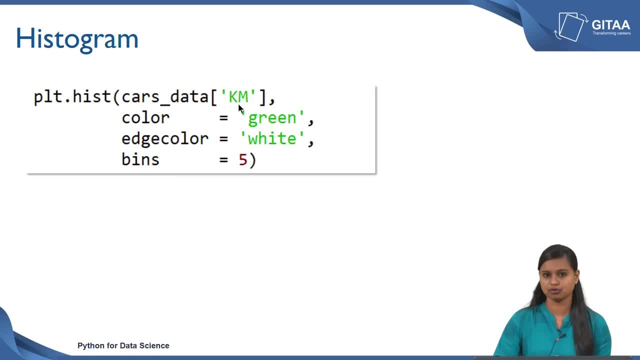 Since we are looking at the frequency distribution of the kilometer of the car and the color for the bars will be green and ah, the edge color of the bars. I am giving it as white So that there is a clear demarcation between 2 bars, and I affixed the number of bins as 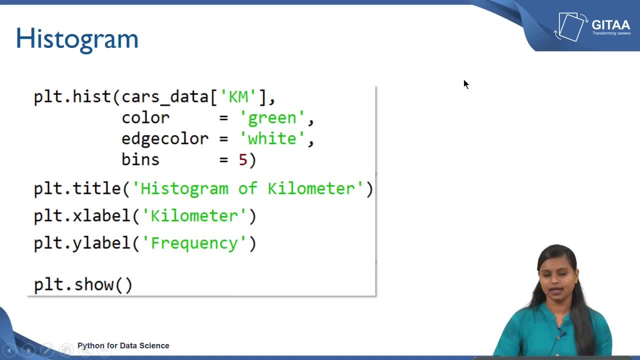 5. And you can also add title x label and the y label to your plot. here the title for the plot is histogram of kilometer and the x label is kilometer and the y label is time. So kilometer and the y label is frequency. and if you give plt dot show and if you run from 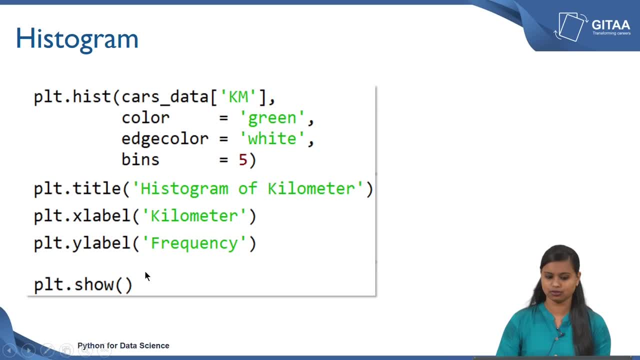 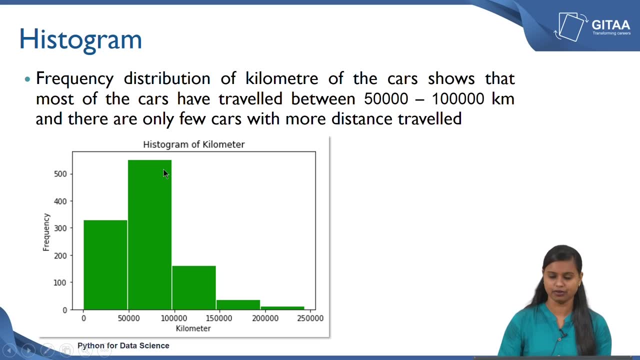 plt dot, hist to plt dot- show you will get a histogram with those specified number of bits. So here is the output that we get from the previous code. So here we are looking at the frequency distribution of kilometer of the cars and it shows that 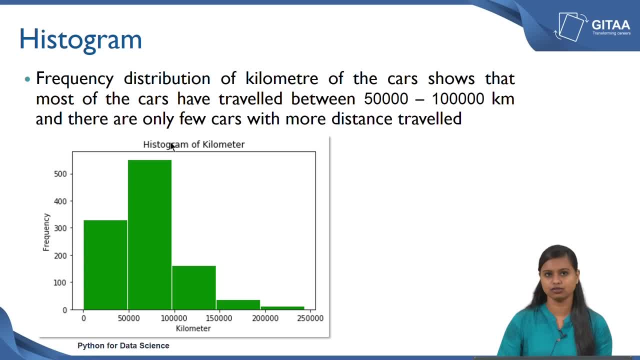 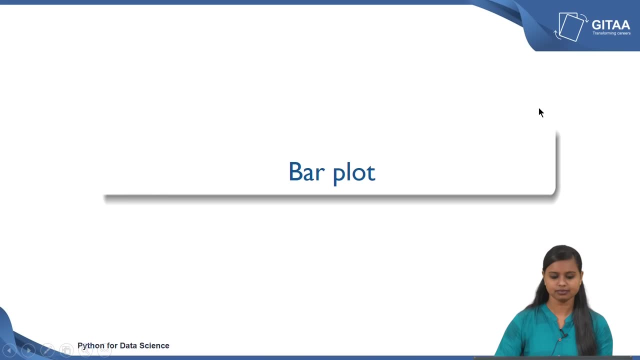 most of the cars have travelled between 50,000 to 1 lakh kilometer, and there are only few cars with more distance travelled. Now, if you see that there is a clear demarcation between each of the bars, and you will be able to look at the frequencies of it easily. 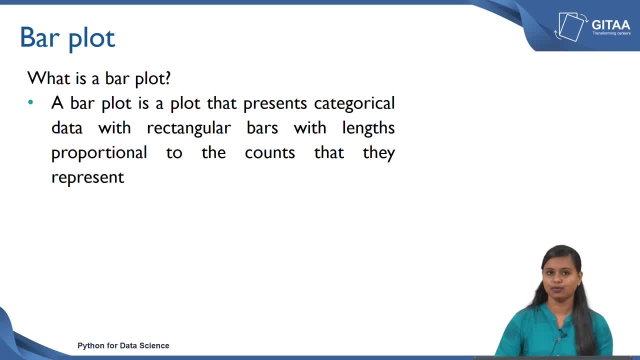 Next, we are going to look at a bar plot. let us see what is a bar plot. bar plot is a plot that represents categorical data with rectangular bars. Whenever you have a categorical data And if you want to look at the frequencies of each categories in a variable, then we will. 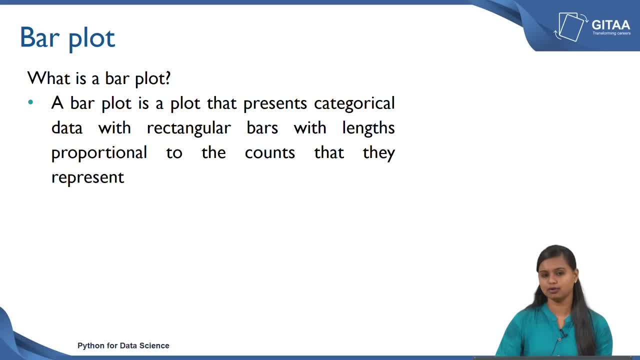 look at in terms of bar plot. Bar plot is also similar to histogram. there would not be any space in between the bars for the histogram because you are looking at in terms of continuous range, But here you will be looking at in terms of frequencies of categories, so you will have 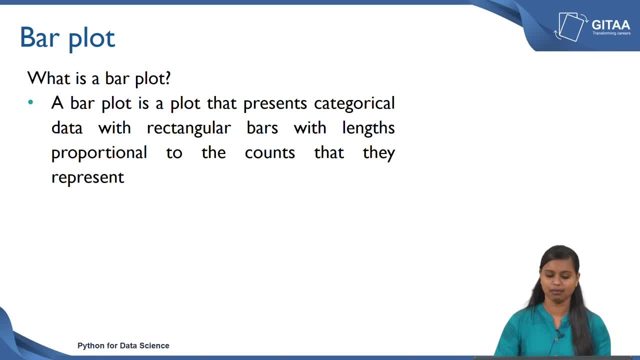 space in between the bars. that is what the difference between the bar and the histogram- and you use bar plot for a categorical variable And we use histogram For a numerical variable- and those length of the bar is basically depicts the frequencies of each categories and when to use a bar plot to represent the frequency distribution of. 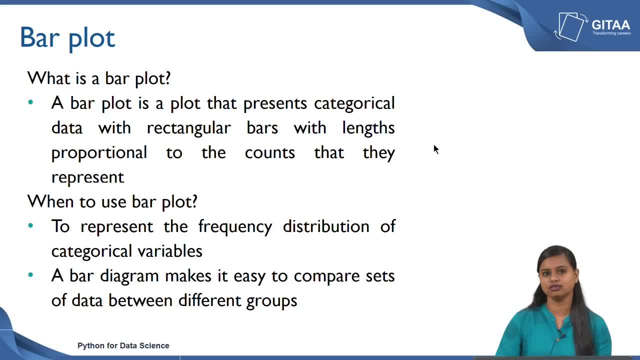 any categorical variables and the bar diagram makes it easier to compare sets of data between different groups. If you have a categorical variable and if you have so many categories under that variable, if you want to look at distribution of each variable or how each category is distributed, 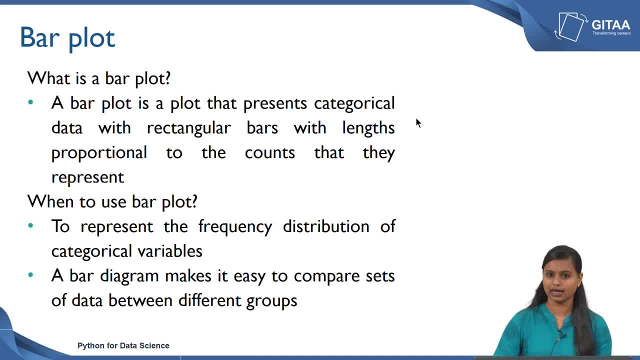 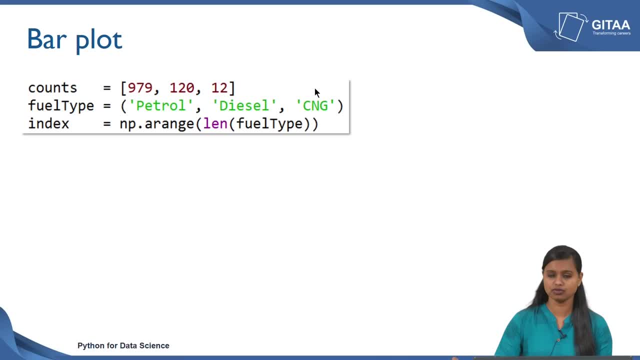 then bar diagram is easier to interpret. more on the categories of a variable. Now let us see how to create a bar plot. Basically, you have to have an array which shows the counts of each categories and the next object or the next variable represents a fuel type. 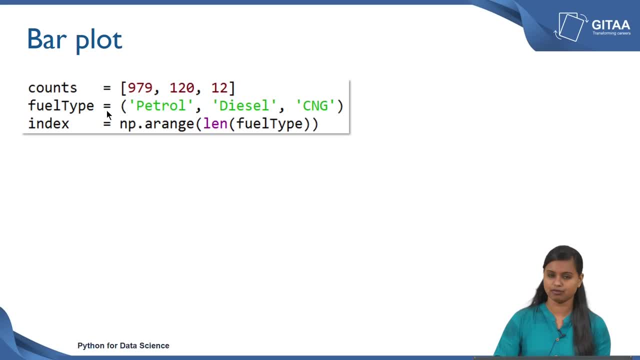 Here we have petrol, diesel and CNG as fuel types of the cars, and since we know that a priori, I have just given. Otherwise, you can also give value and the score counts as well. So that is what we are going to do. 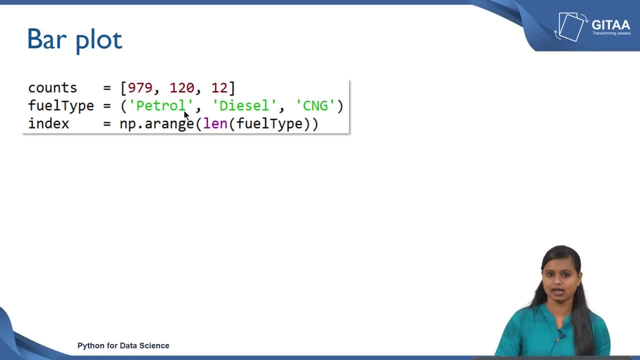 Thank you. So that is what we are going to do, Because that will have the category as well as the frequencies, and I have given index because on the x axis it should know the index. The index is: whatever is the length of fuel type. what is the length of the fuel type? 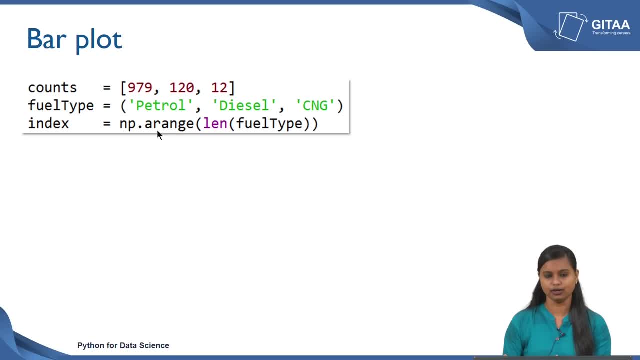 it would be 3.. So the range would be 0,, 1 and 2 and to create a bar plot, that bar is the function that is from the pipe plot sub library, and inside the function you just basically need to give value: what should be there in the x axis and what should be there in the y axis and x axis. 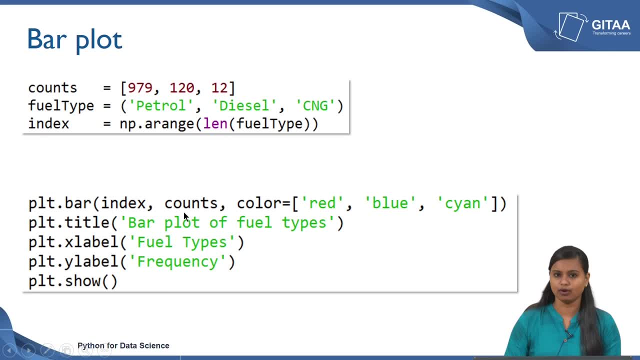 I want the index to be present and on the y axis, I want the counts to be present, and I am going to color my bars differently: red will go for petrol, and diesel will be colored based on blue color and CNG will be colored based on CYA and color. 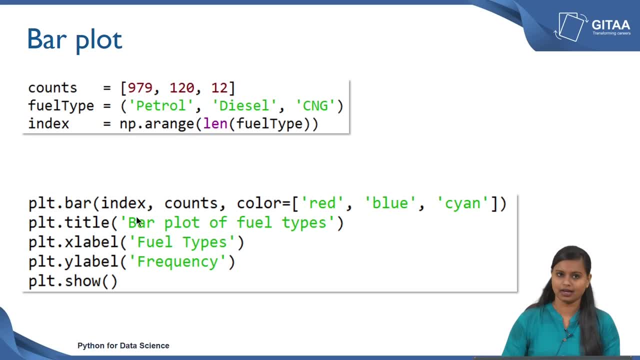 And I have also given the title and the labels for x and y axis so that I can create a bar plot Which will show the frequencies of the fuel type categories. And, as I have mentioned earlier, x index is nothing but x coordinate and count will represent. 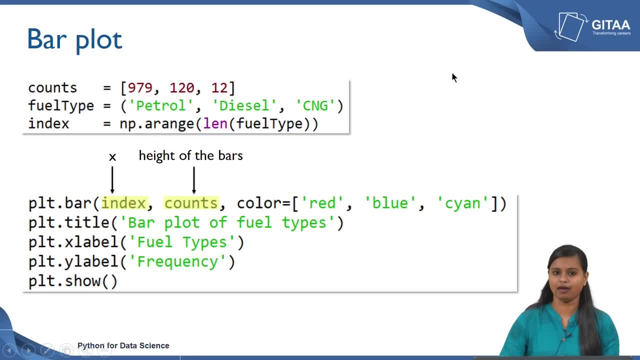 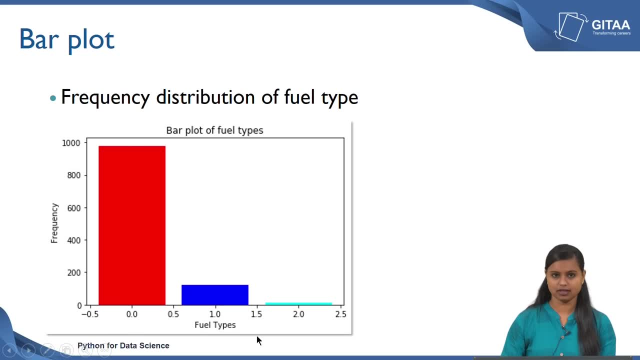 the height of the bar, and height of the bars have been represented using counts. So this is the output that we got. but if you see, on the x axis you have only the range. here we are not able to find out which is petrol, which is diesel or which is fuel. 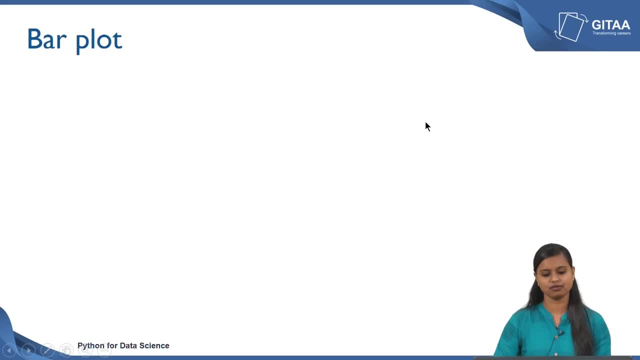 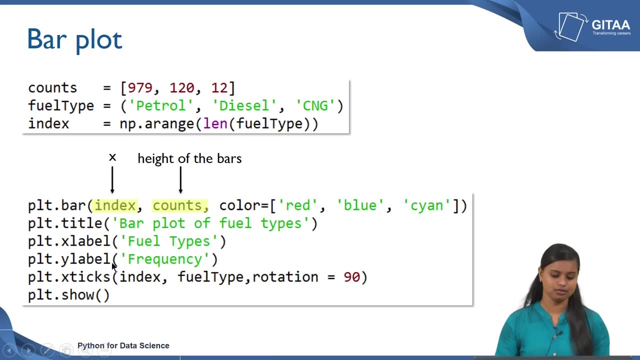 So this is the output that we got, Which is CNG. In that case, you can also specify the labels to your x axis by giving x ticks. So all the other codes remains the same, but since I just want to add labels to each, 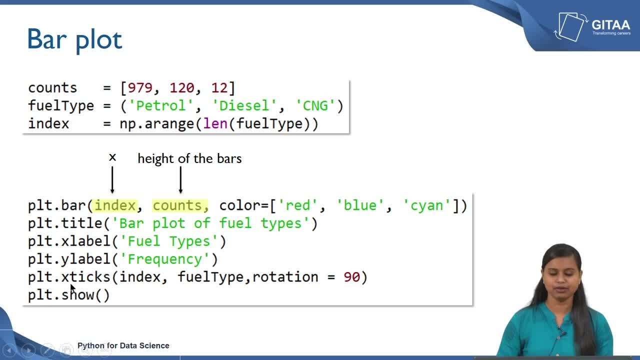 of the bars on the x axis that can be given using x ticks. You can set the labels of the x ticks using fuel type because you have already assigned the variable called fuel type with some string values. So that will be labels for the x ticks. 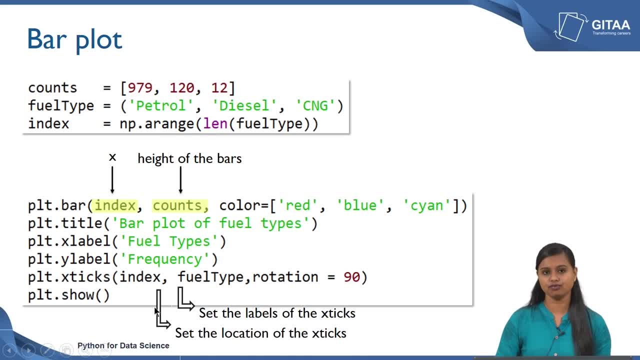 So that is the output that we got. So this is the output that you can get using fuel type. Here you also set the label for x ticks. You can also set the location for x ticks: Where petrol should be present and diesel should be present and CNG should be present. 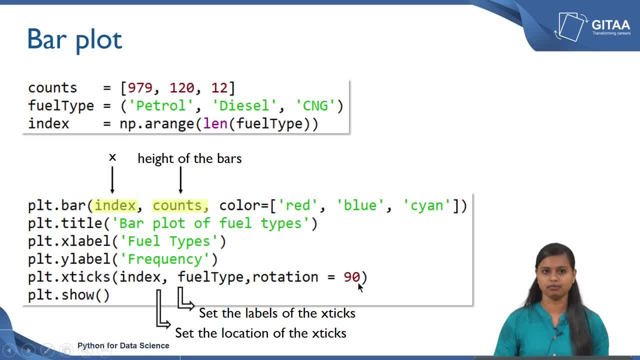 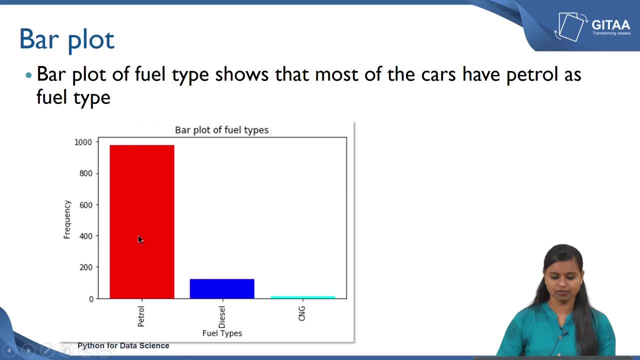 And I have given rotation is equal to 90, so that all the labels will be in 90 degree rotation. So now let us see how the plot will look like Here. if you see this, the first bar is corresponding to the petrol fuel type, and it is very evident.